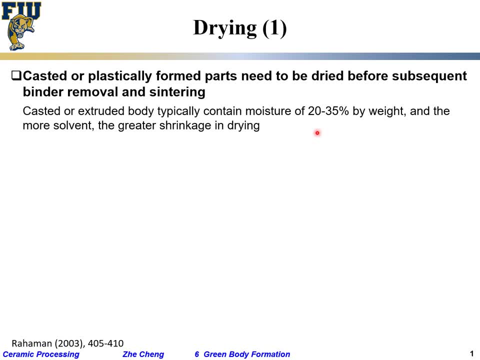 percent of solvent by weight, And the more solvent, the larger the solvent, the more larger the shrinkage just by the capillary force. okay, Here we see typical drying depending on how much moisture or solvent content. sometimes it has so-called multi-stage drying Here. 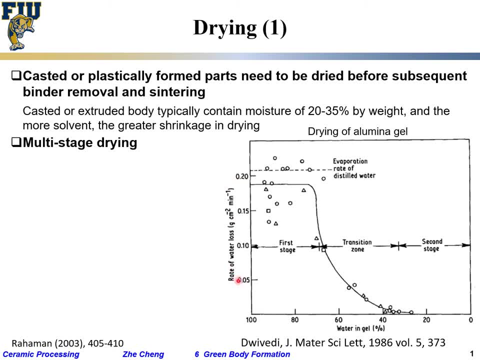 I'm showing a multi-stage drying. The vertical axis is rate of water loss. It's essentially how fast the solvent leaves You are green body. The horizontal axis is water content in your so-called body, green body right. So initially, when the water content in your gel is high- of course not 100 percent. 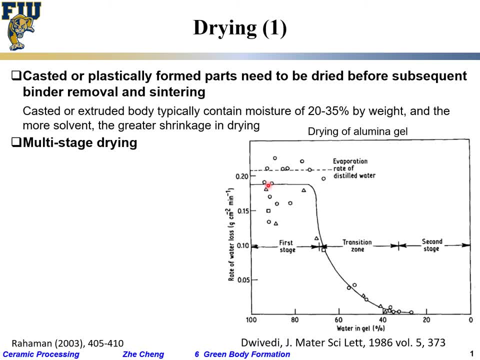 high, high. your rate of water loss would be initially high, but then, as you have less and less so-called water content in your gel, you have less and less water content in your gel. the rate of water loss would naturally decrease. Make sense: You are getting drier. 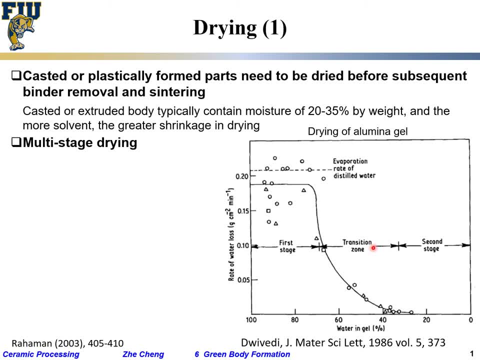 and drier, of course, the rate of losing water become lower and lower. So this state people can call so-called constant rate period or CRP. okay, Liquid essentially covers almost the entire body. Okay, Okay, Okay, Okay, Okay. 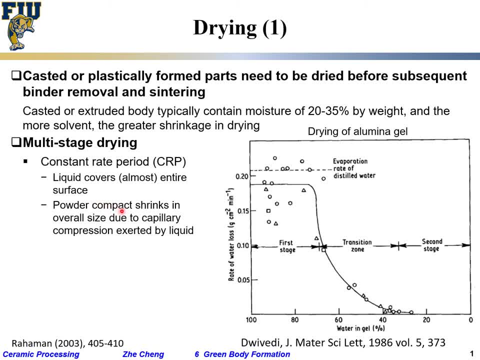 Okay. Okay, It dries relatively fast. Powder compact in this state would shrink in so-called overall size due to capillary force. The water is lething. it's pulling everything together with it so that every powder come exerted by the liquid Make sense. 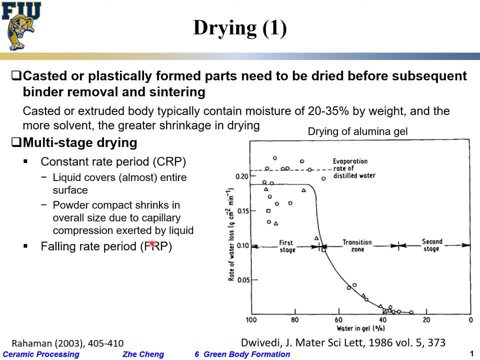 And then so-called falling rate period. FRP. falling rate period period. the moisture content or solvent content is much lower and quite often there would be no further reduction in compact size because after a certain point the powders would start. 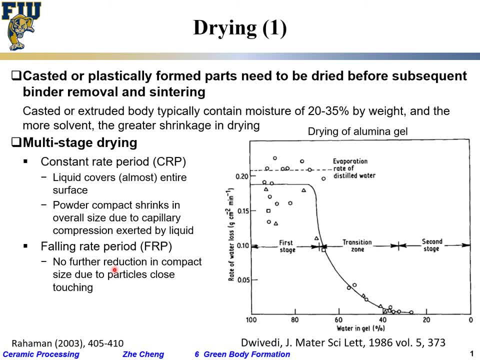 to already touch each other Without sintering. just by solvent removal you cannot make the particles pack denser. Make sense. So not much further reduction in compact size because the particles are already touching each other, unlike they are suspended in the slurry or 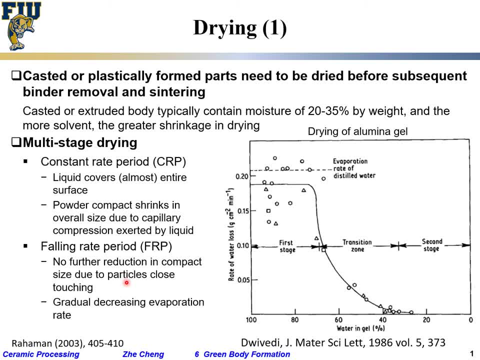 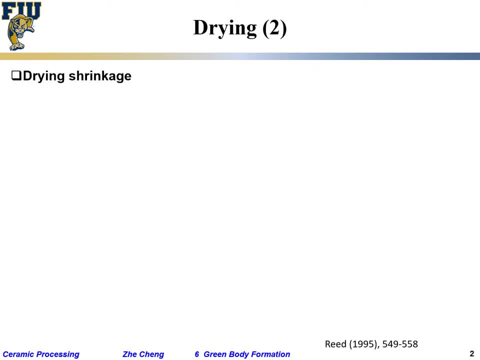 suspension Make sense And then there will be a gradual decrease, gradual decrease in evaporation rate. Okay, The drying shrinkage is very important. Here we are showing the volume shrinkage versus moisture content, assuming we are using water as well as soil. 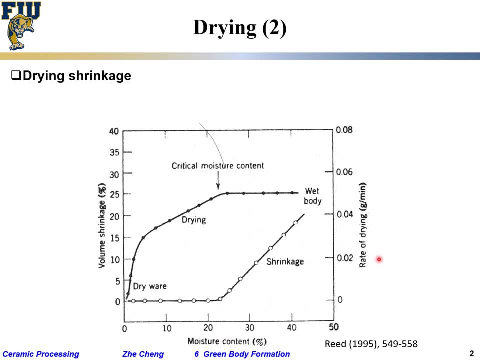 and sand. rate of drying, which is how fast we are removing water, versus the moisture content. let's first look at the shrinkage curve. shrinkage curve- if which is this way right- shrinkage shrinkage, volume shrinkage: if the body has more moisture, it would have higher shrinkage. on the other, 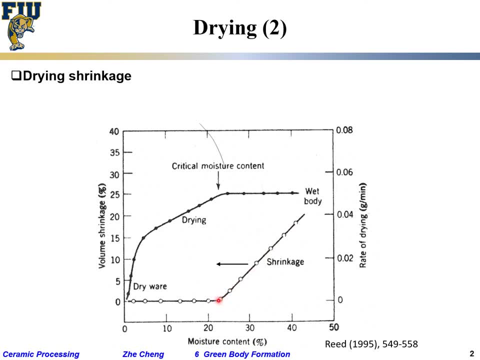 hand, when the moisture content decrease, decrease, decrease to certain points. the shrinkage beyond that would be very small, because beyond here, essentially each individual particles are already packed, reasonably dense, and further water leaving the system, moisture leaving the system. it's just that they're arriving away from the pores. you cannot cause the. 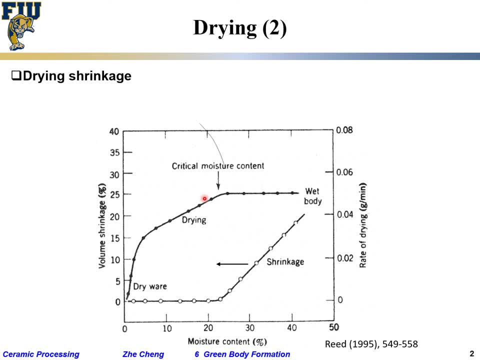 particles to come any closer make sense. that's not enough driving force. the shrinkage is larger when the solvent content is higher than roughly 20 percent. make sense. the shrinkage is small or essentially no when the solvent content becomes less than roughly. this point because they are. 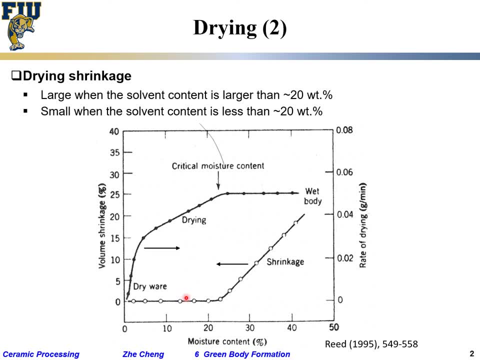 essentially particle touching, and the other side is about rate of drying. rate of drying when the- not surprisingly, when the moisture content is high, your rate of drying is. here you are reading towards the right side. the rate of drying is fast and your moisture content decrease. the rate of 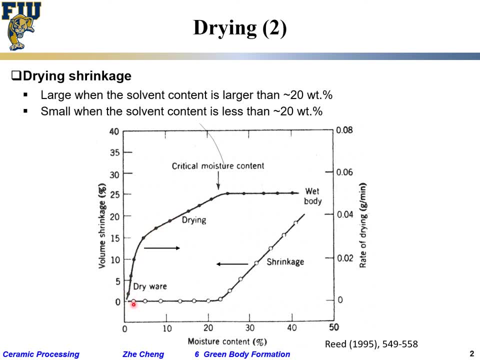 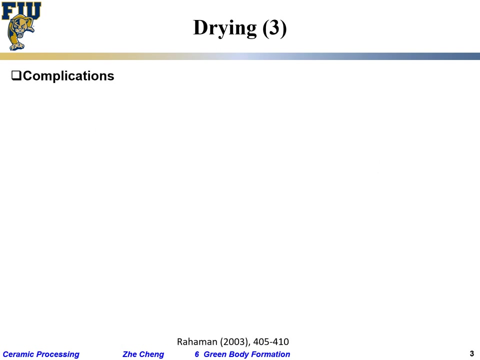 drying also decrease. towards the end you have very little moisture. your rate of drying, which is how fast you are removing solvent, gram per unit time decrease almost to zero because you do not have much solvent left. make sense, okay. and then drying. if you ever handle ceramic, you'll find it's. 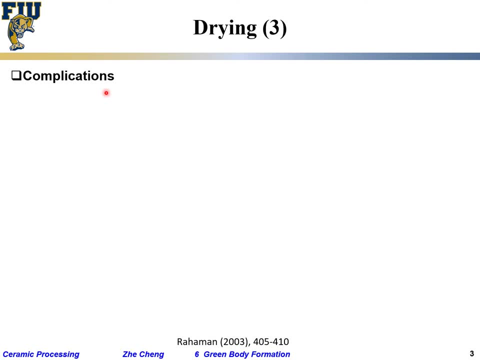 a lot of complication. looks simple, just like when you cook. looks simple, but sometimes you have all types of defects: capillary action in drying which, if not controlled well, may lead to non-uniformity or severe cracking in your green body. okay, here we are giving the schematics. 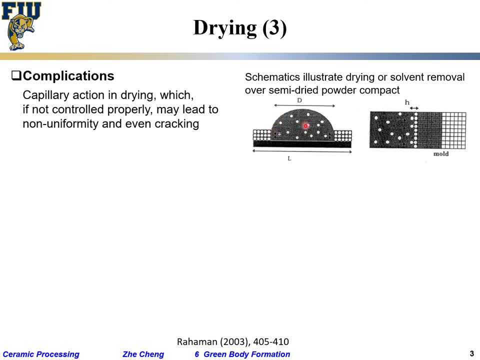 we have the ceramic body, but then some portions do have liquid. some portions have kind of like semi-dried, have solvent in between them and you can imagine the solvent in this bead of slurry will evaporate at one time, at the same time, if they are going to suck into the neighboring. 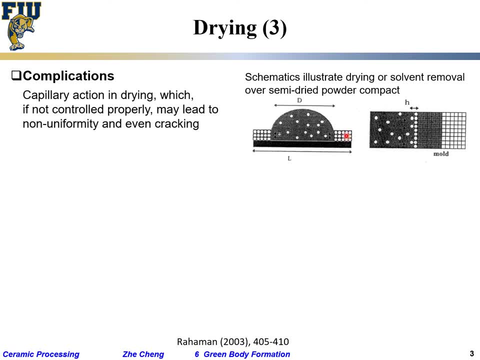 dried region and that capillary force can be significant. okay, if not controlled well. and similarly, if we have mold, if we have slurry or suspension at a surface, we would have particle packing and the solvent would continue to migrate or suck into the mold. and if we are not controlling it well, the capillary force can cause cracking. 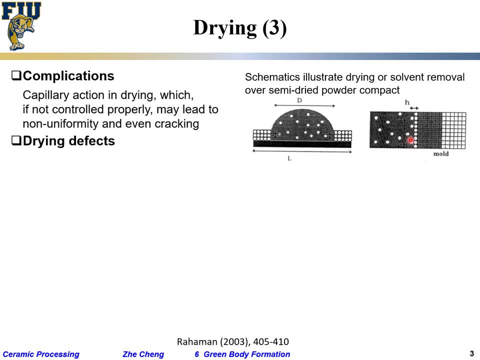 in the sediments, the drying defects, deformation such as bending, which can come from all types of unsymmetric symmetry or non-uniformity. here we have higher vapor pressure on one side, lower pressure on the other side. it may cause to burn. we have finer particle on one on the top.